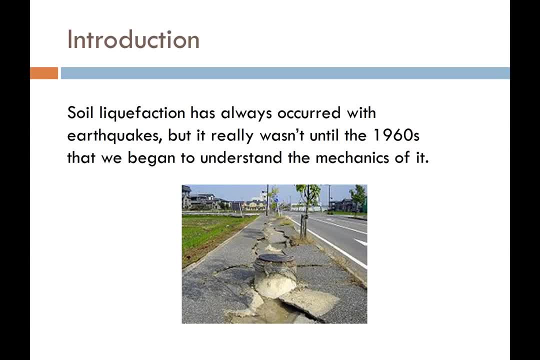 in the 1960s we had a lot of earthquakes, And so in the 1960s we had a lot of earthquakes, And so in the 1960s, a huge push to understand and perform research on soil liquefaction began. 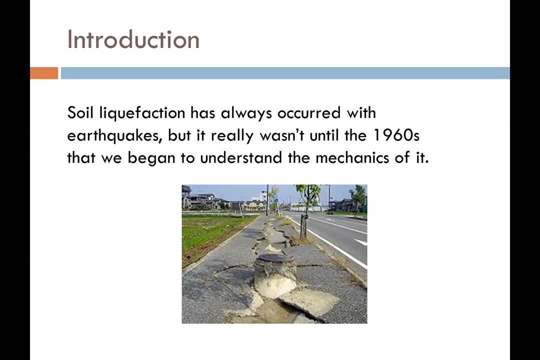 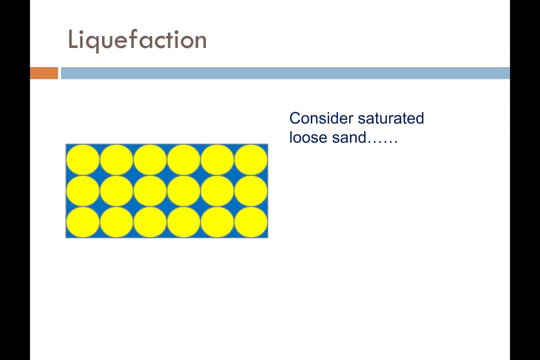 And it really is kind of the baseline, I guess, or the fundamental principles, of what we're going to talk about in this lecture. So since the 1960s we've learned a lot about the mechanics behind soil liquefaction, And so let's review some of those right here. 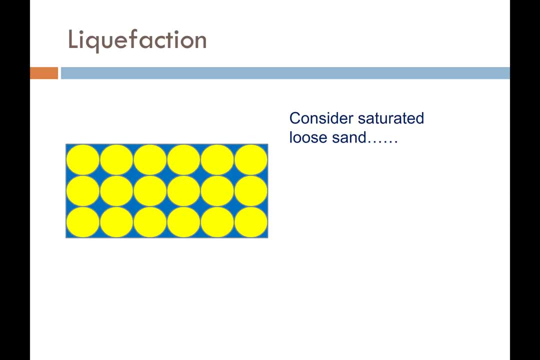 Now if we had a saturated, loose sand, as this little cartoon here shows? Now we know that the sand is loose because you can see, the void space in between the sand particles is very, very large. If the particles, if the sand particles were any closer together, the void space in between the sand particles would be smaller. 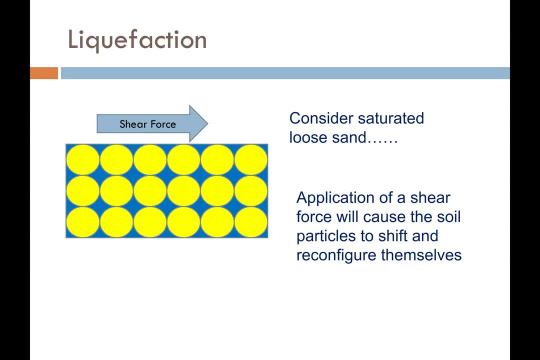 Now, if we apply the shear force to these sand particles, it's gonna force these sand particles to rearrange and reconfigure themselves relative to one another. So you can imagine that this row of sand is going to slide this way and this row of sand 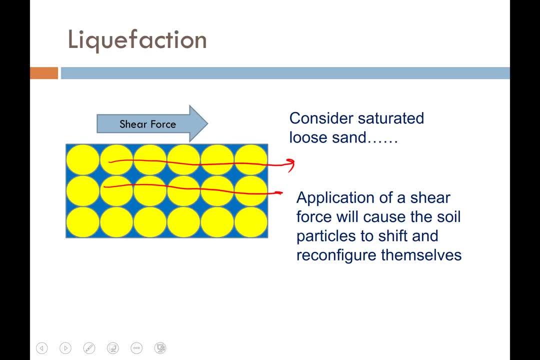 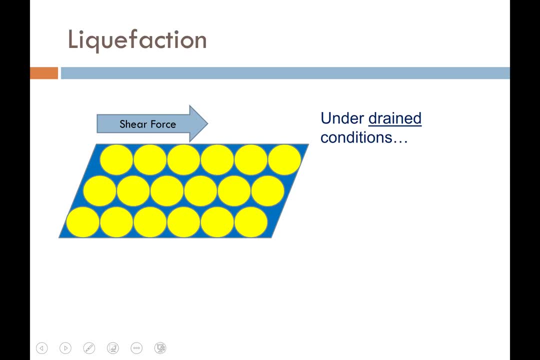 might slide a little bit that way And the result is going to look something like this: Now, if I pause the entire mechanism in the process, all I did was I smoothed the sand particles over to the right. Now if I have drained conditions. 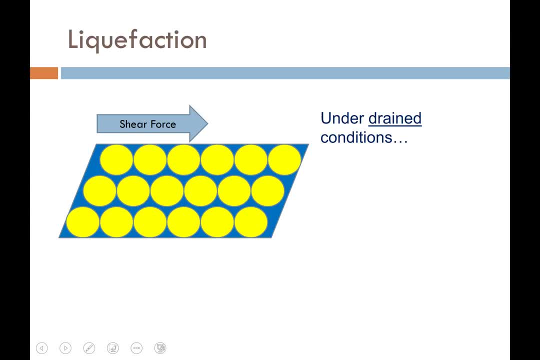 what's going to happen is these sand particles are going to try to settle and come back into contact with one another and they're going to push the water out of the way. And the water can get out of the way because it's a drained condition. 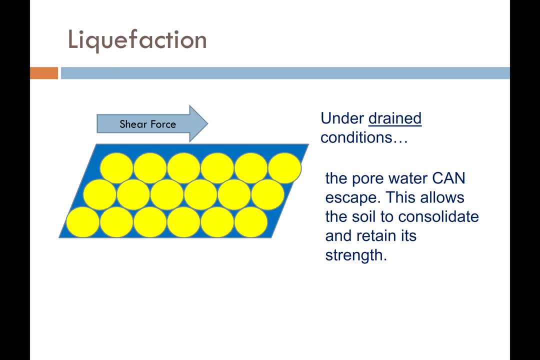 Because it's drained. the water can get out easily, and what ends up happening is the ground settles and we have a compaction, so to speak, or a consolidation, But once the particles come back into contact, they've regained their strength. 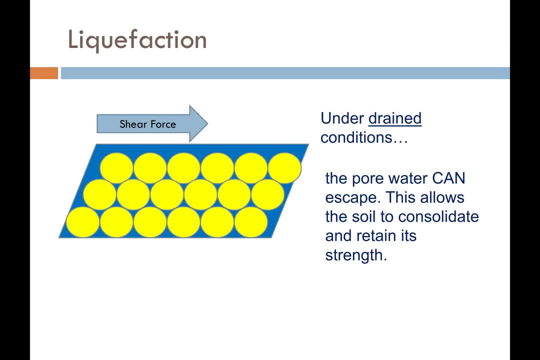 They've regained strength again and the soil is dense and stiff. Now let's reset If our particles are suspended again in this manner. but we have undrained conditions, meaning that the sand particles want to settle down. they want to consolidate down into the void space. 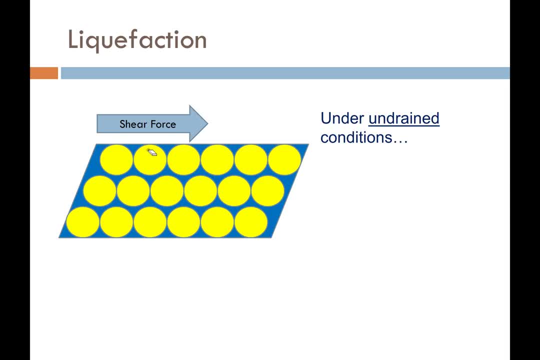 the problem is that the water's in the way, There's nothing, and because it's undrained, there's nowhere for the water to go. So, as a result, the water pushes back And because the pore, water can't escape. 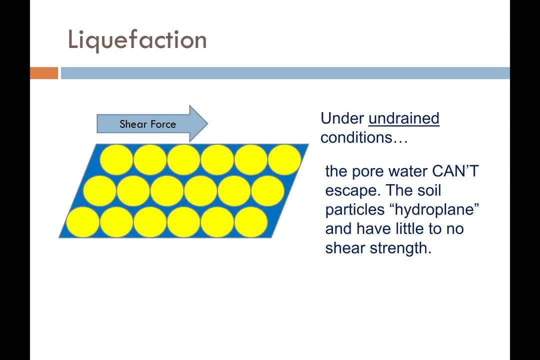 essentially, then, the soil particles hydroplane on the water, that's, in the void space, And for a very temporary period the soil particles have, or the soil itself has, very little to no shear strength. So it's important to remember that this is a temporary. 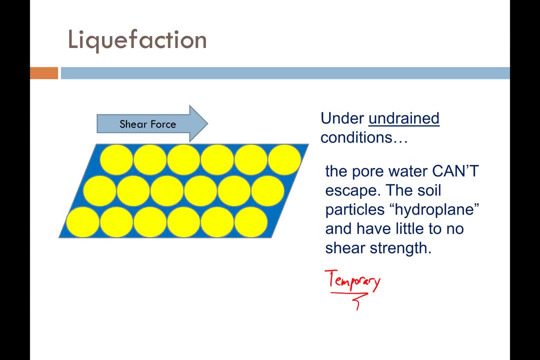 condition because, remember, this is a loose sand. Yeah, Yeah, Yeah, Yeah. And when we think about undrained soils, we think of clays or the things with low permeability, And the reason that it's this way in sand. 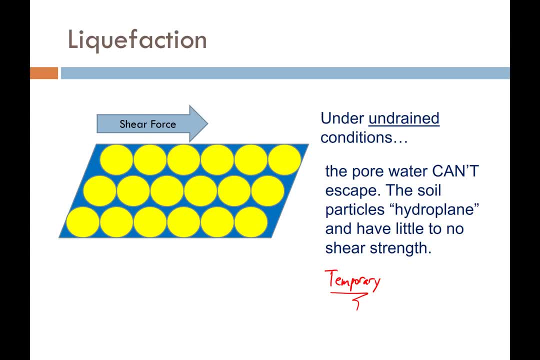 is because all of the sand is trying to compact itself and squeeze the water out simultaneously at the same time, And because all of the water's trying to get out at the same time, it can't do it fast enough, And so there's a backup. 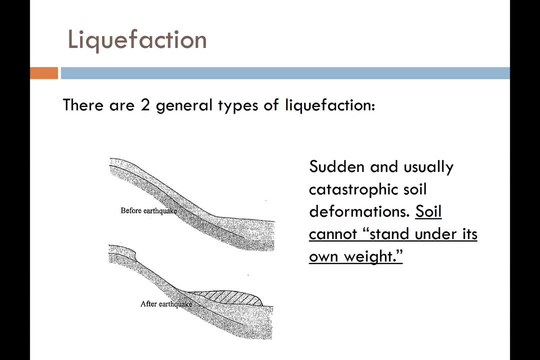 And as a result of that, we get the undrained condition in sand. so that's the basic mechanism behind liquefaction. now let's zoom out and let's look at liquefaction from a larger or a higher elevation. there are essentially two general types of soil liquefaction. the first type is: 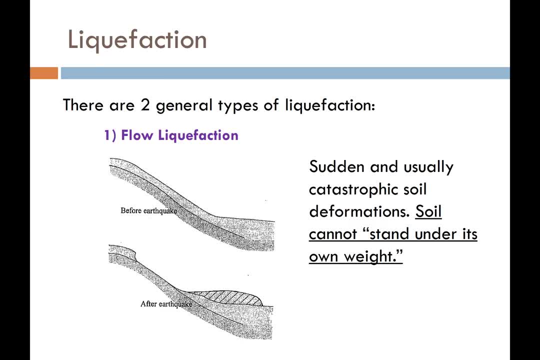 referred to as flow liquefaction, and flow liquefaction is characterized by a sudden and a usually a catastrophic soil deformation. so let's say that this whoops, let's say that this soil here on the slope liquefies, and because it liquefies, it can't hold itself up under its own weight. so because of that, that 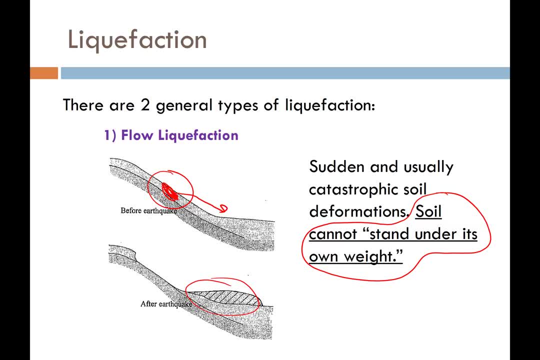 soil is going to flow down slope like this and we can get some tremendous ground deformations and you know this is the type of effect that we're going to see in the next few slides. so let's zoom out and let's look at that. can really cause some damage and can hurt people, because it happens very. 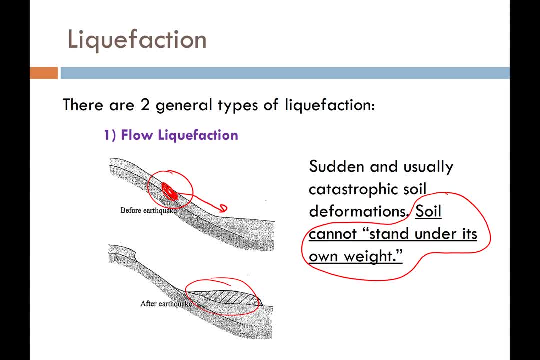 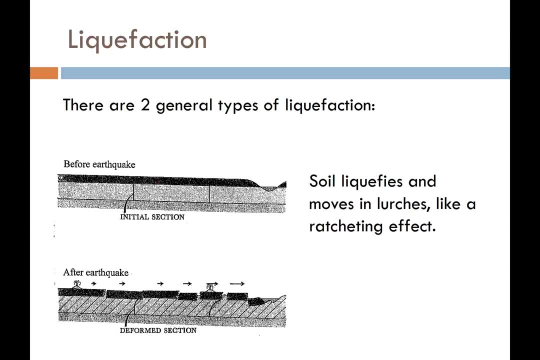 quickly and usually without warning. now the second type of liquefaction is not as dramatic, but certainly can be just as damaging to infrastructure, and it's called cyclic mobility. now, in cyclic mobility, the soil liquefies and as it liquefies and the ground, motions are still occurring that are going to shake the ground back and forth. what ends? 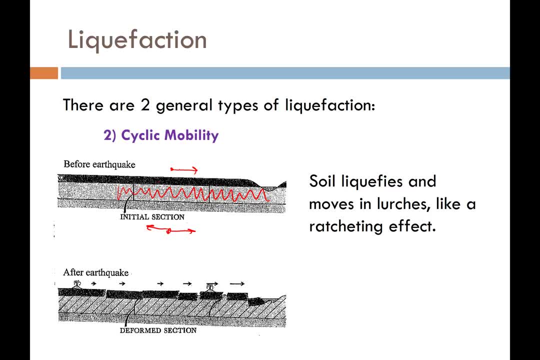 up happening is the soil also begins to lurch back and forth on top of this liquefied soil and if there's anything like an open canal, or if there's a gradient or the slope in the ground, the every time we get some ground motions, we 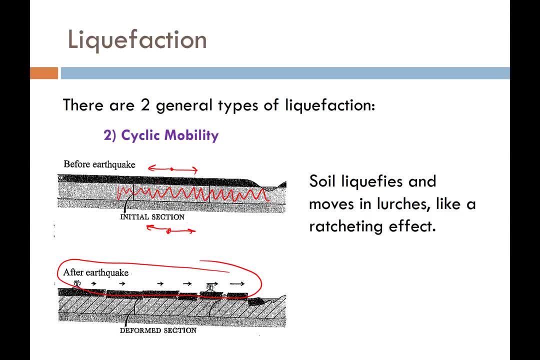 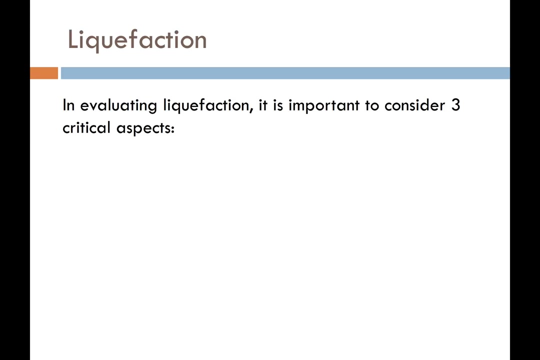 may end up actually seeing permanent deformations and cracking in the ground, and which can lead to an effect known as lye- lateral spreading. so cyclic mobility can result in significant ground deformations, but they're just not as dramatic or as sudden as flow liquefaction. so whenever we talk about or address the topic of liquefaction, 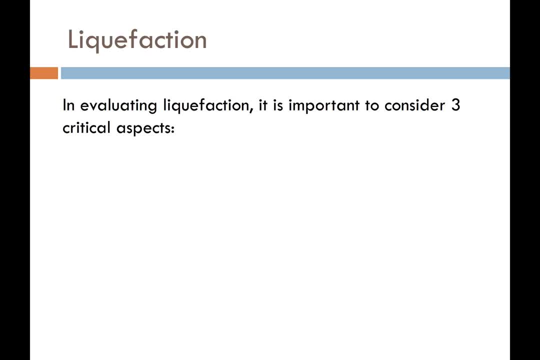 there are three critical aspects that we need to consider. the first critical aspect is susceptibility of a particular soil to undergo liquefaction. the second is liquefaction initiation. if my soil is susceptible, will it liquefy under a given level of ground motion? ground motion, then. the third question is: 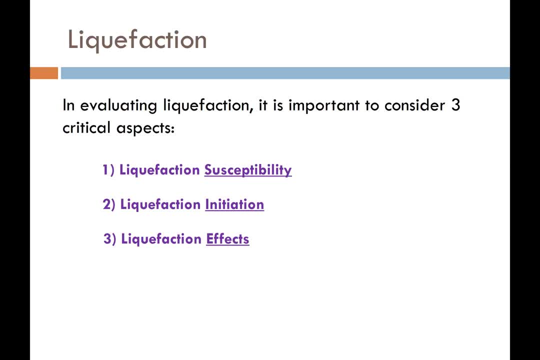 the effects. so if my soil is susceptible and I do predict that it will liquefy under the design ground motions, what are going to be the effects from that liquefaction? and so if we frame the problem of liquefaction in this light, with these three critical questions, are things that we need to address. we can be. 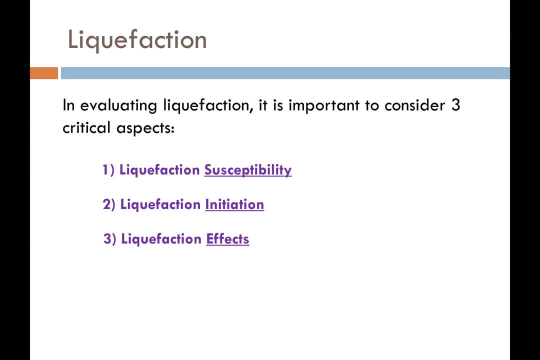 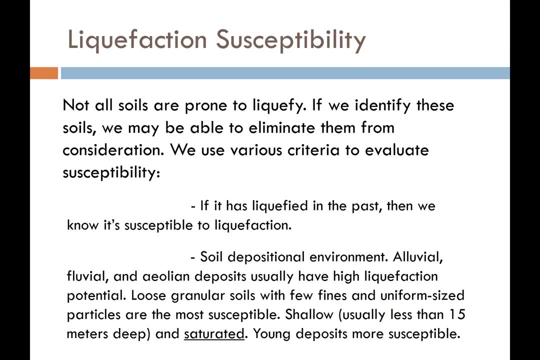 objective and repetitive in the way that we analyze liquefaction. let's talk first about liquefaction susceptibility. now we know. we know that not all soils are prone to liquefaction. now we know that not all soils are prone to liquefaction, to liquefaction, and we can- if we identify these soils ahead of time, we can wave our magic wand. 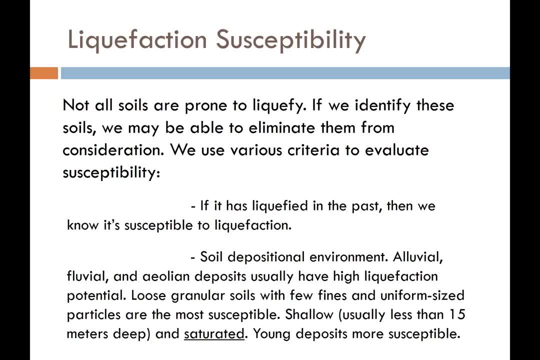 and remove them from the analysis and so that they won't contribute to the problem, and there's different levels of criteria that we use to establish susceptibility. so, for instance, if there's evidence that liquefaction has occurred at our site at some time in the past, then that's kind of a deal killer. we know right off the bat that liquefaction is likely and 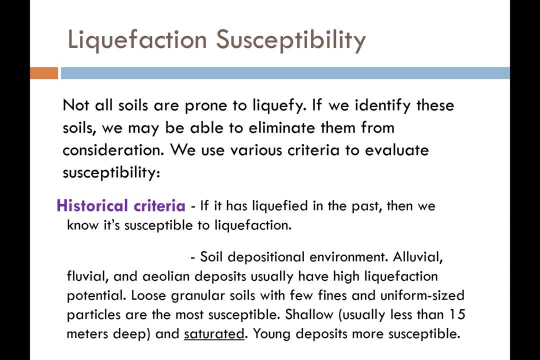 probable to occur in the future. so liquefaction tends to occur in the same places over and over again. it tends to repeat itself, and so if a site has liquefied in the past, then we know it can have great confidence it will probably liquefy again in the future. another criteria that we use is: 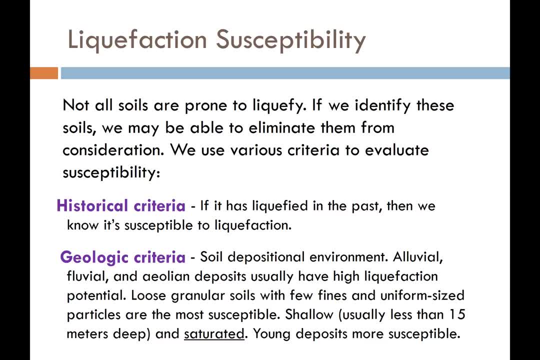 liquefaction, called geologic criteria, and this is an important one, and it's often overlooked by engineers, though in my opinion it shouldn't be. we know that certain geologic depositional mechanisms lend more to liquefiable soils than others, so, for instance, we know that soils that are 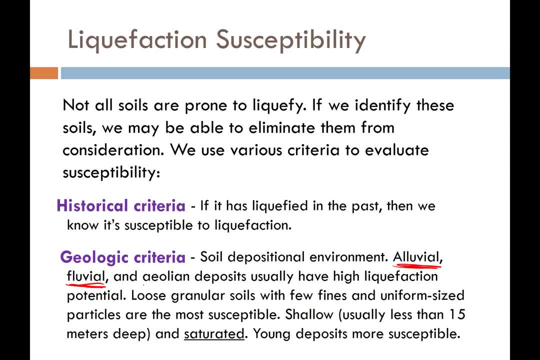 deposited alluvially or fluvially or aeolian, like through wind action, that that those types of deposits tend to be more likely to be liquefied than others, and so we know that deposits tend to be the most susceptible to liquefaction. we also know that soils that 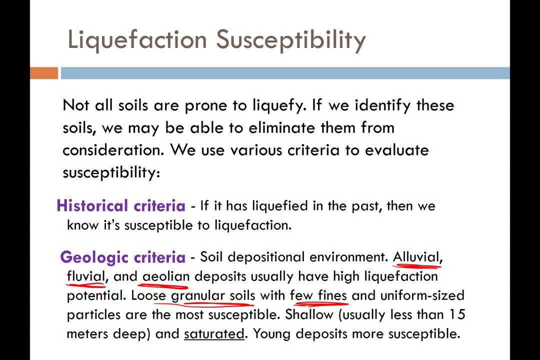 are granular in nature, that have few fines and that are uniform in their size and their particle distribution are also they also tend to be more susceptible soils that are shallow, you know, usually less than 15 meters below the ground surface, and preferably less than 10 meters. 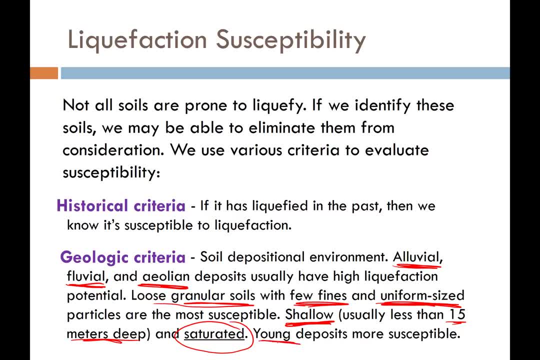 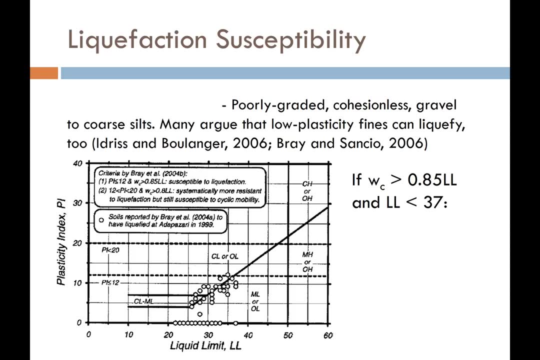 and that are saturated and that are young, so relatively recent, particularly deposited in the last last 10 000 years. those types of soils are the most susceptible to liquefaction. another type of criteria is called the compositional criteria, and compositional criteria. it looks at the type of the soil. 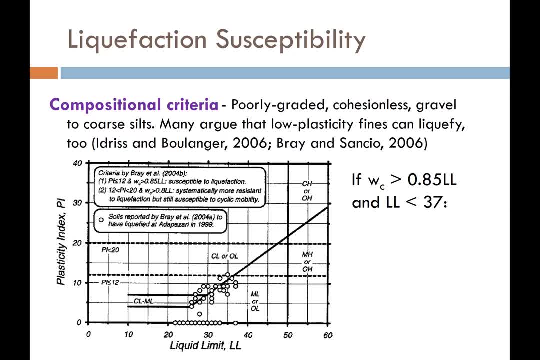 not how it was deposited or how old it is, but which is really like what the classification or the type of the soil is. we know that poorly graded, cohesionless and gravel to core silts are the most likely candidates for liquefaction. however, we've learned in the last, i would say, 11 years or so that many low plasticity fine soils 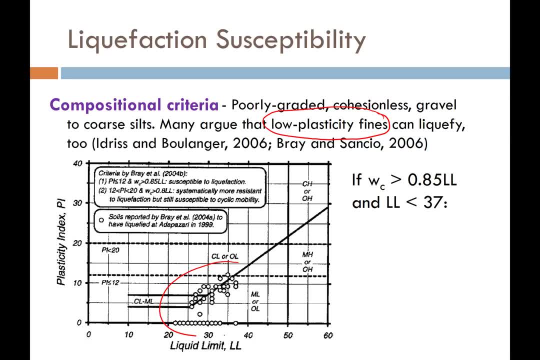 can also liquefy, for instance. you see this plot down here. this comes from. looks like this one is probably out of taken from a publication of Boulanger and Idris and it talks about the different criteria. Now, Bray and Sancio 2006, recommended that anything less than a plasticity 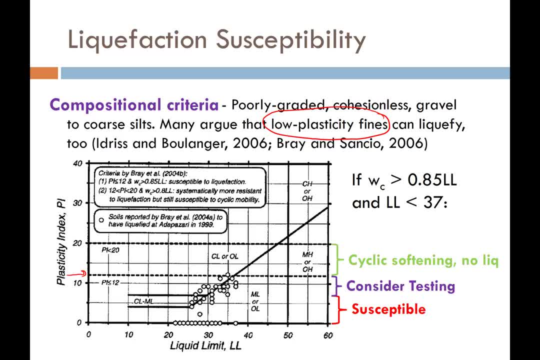 index of 12 should be considered susceptible to liquefaction, And it also has to have a water content greater than 85 percent of the liquid limit and the liquid limit needs to be less than 37 percent. If those criteria apply, then Bray and Sancio say yes, Assume that the soil is. 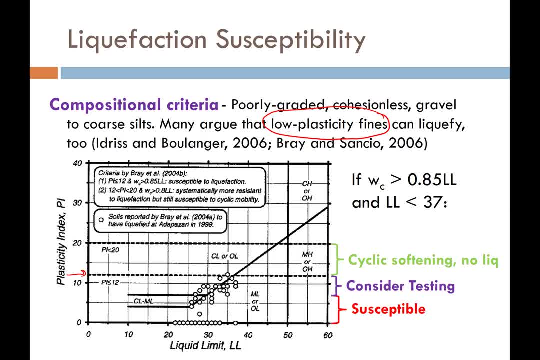 susceptible. Now, Idris and Boulanger, they take a little less conservative approach and they say no, the line should be somewhere around a PI of seven. So if your less, if your plasticity index is less than seven, and these criteria apply, 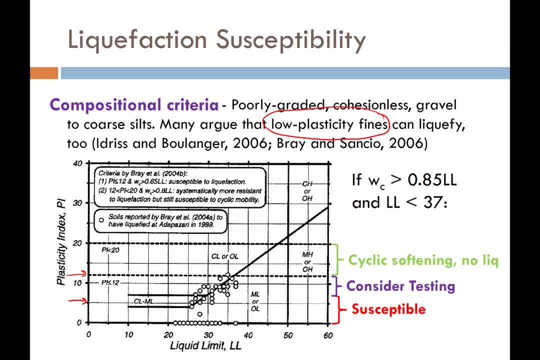 then yes, you should consider your low plasticity fine soil to be susceptible to liquefaction. Now there's a lot of argument between these two camps. Is the plasticity index 12 or 7?? 12 or 7?? And really I think that what has been decided is that if your soil falls within this, range, then you should consider your low plasticity fine soil to be susceptible to liquefaction. Now there's a lot of argument between these two camps. Is the plasticity index 12 or 7?? 12 or 7?? And really I think that what has been decided is that if your soil falls within this range, 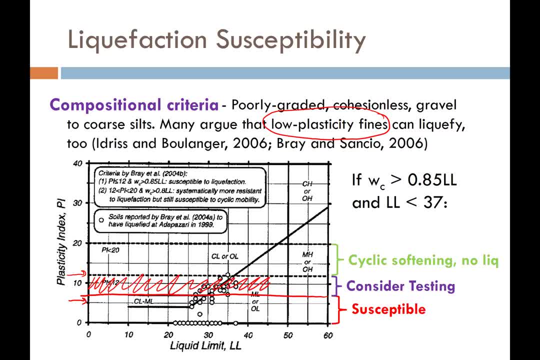 between a plasticity index of five or seven and 12, that maybe you consider testing it in the laboratory to see if, under the design ground motions that you're anticipating for your site, if it will liquefy. Now, another type of susceptibility is what we call the state. 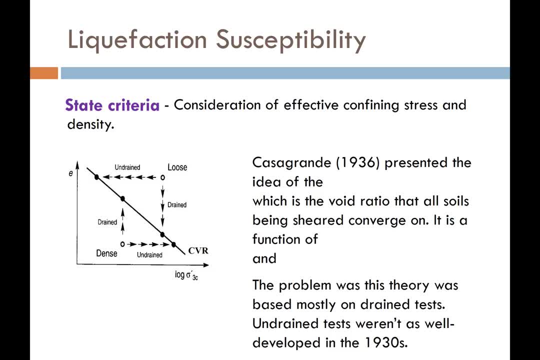 criteria. The state criteria has to do with whether or not the soil is susceptible to liquefaction, So what we call loose or dense. Now, loose soils tend to liquefy, Dense soils tend to dilate and not liquefy. Now the late professor Arthur Casagrande, in 1936, presented a very critical idea. 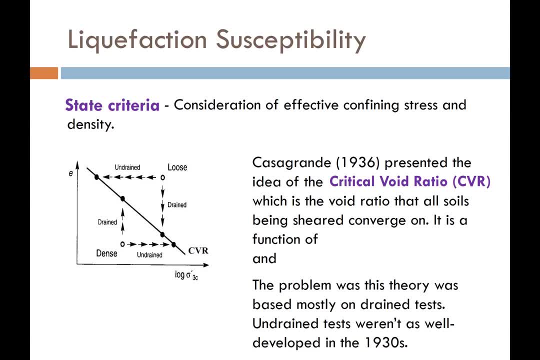 called the critical void ratio And, according to this theory, Casagrande stated that all soils, regardless of whether they're dense or loose, when you try to shear them, the soils try to make their way to a line that he called the critical void ratio line. 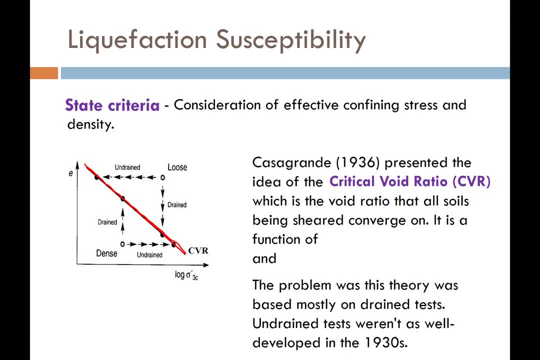 And it doesn't matter if you shear the soil in a drained manner or an undrained manner, that the soil is going to try to make its way to that line. So, for instance, if I have a dense soil and I'm draining it, I'm going to try to make its way to that line. So I'm going to try to make its way to that line. 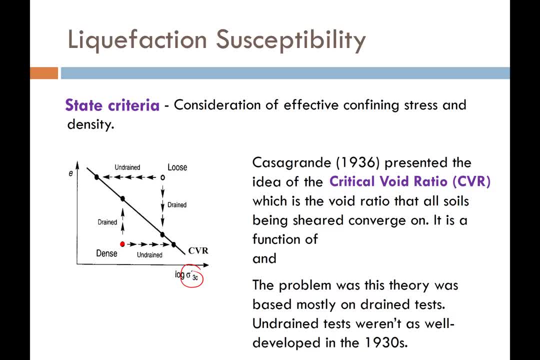 If I'm doing it in a drained manner, that means that my confining stress is not going to change, because I'm not adding any additional pore pressure during the loading, because the test is drained. But what's happening is I'm allowing the volume of my soil to change and the void ratio to change. 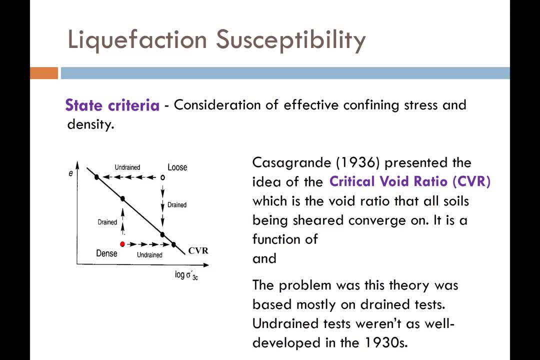 along with it. If my point is here and I'm keeping my stress constant, that means that my point has to go up to eventually reach the critical void ratio line. If it's going up, that means that my void ratio is increasing, which means that I have dilation. 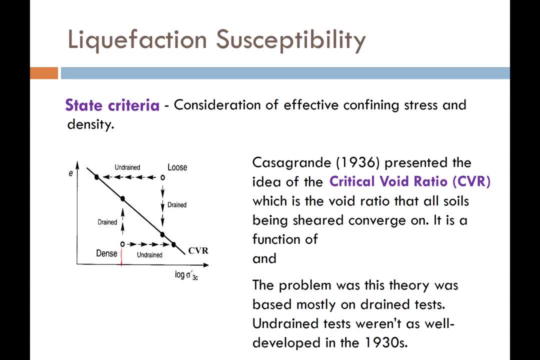 So my soil is expanding in its volume. Now, conversely, if I have an undrained test- and I'm still testing that same dense soil, undrained means that my void ratio is not going to change. I'm going to have constant volume during my test. 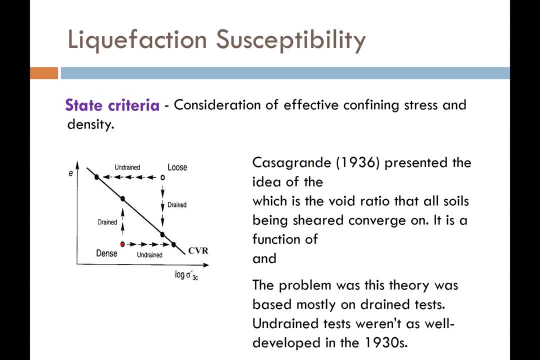 That also means that I'm going to generate excess pore pressures during the shearing action in the test. Now, if my point is here, the only way it can get to this line without changing volume is to go straight over to the right. So if I'm going straight to the right, that means that I'm gaining effective stress. 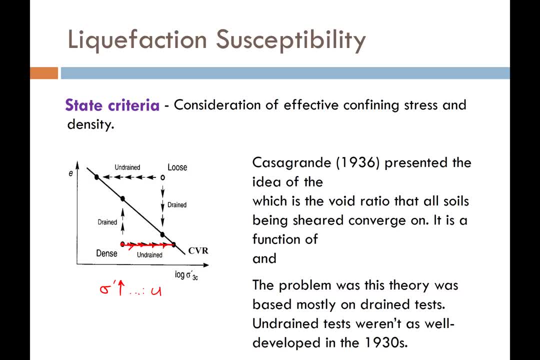 If I'm gaining effective stress, that means my pore pressure is going to be negative, because we know that effective stress equals total stress minus pore pressure. So if I have a negative pore pressure and I'm subtracting a negative pore pressure, I'm going to get an increase in my effective stress. 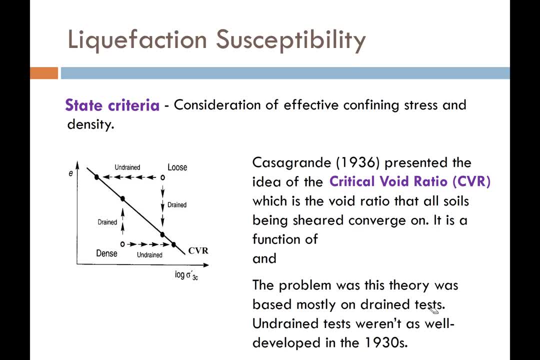 So, again, that's due to dilation. So this theory then of the critical void ratio: it's a function of both the effective confining stress and the initial void ratio. So, regardless of where my soil is, If my soil sits relative to this critical void ratio line, it's going to tell me whether 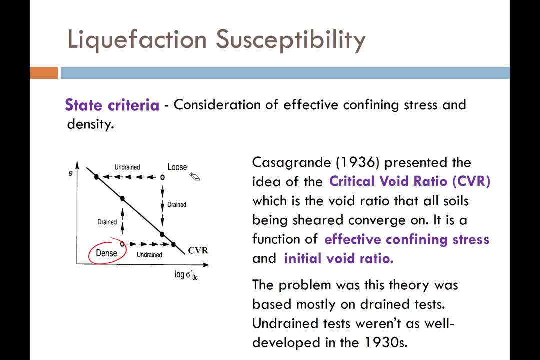 or not I have a loose soil or a dense soil. If my soil sits above the critical void ratio line, it's a loose soil and it's considered susceptible to liquefaction. Now, this theory was widely accepted in the early 1930s and mid-1930s. but there was a 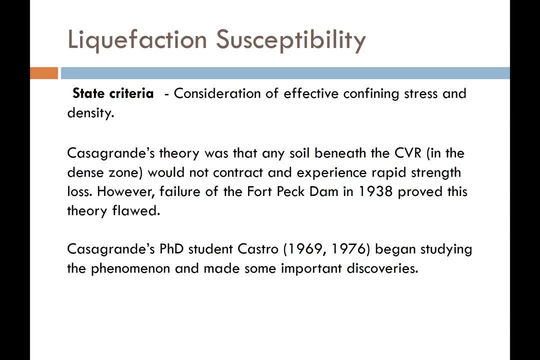 problem with it. The problem was that the Fort Peck Dam in 1938 fell And it was designed based on this theory, And it fell due to liquefaction, And this remained a mystery for a few decades, until later, Casa Grande's PhD student Castro. 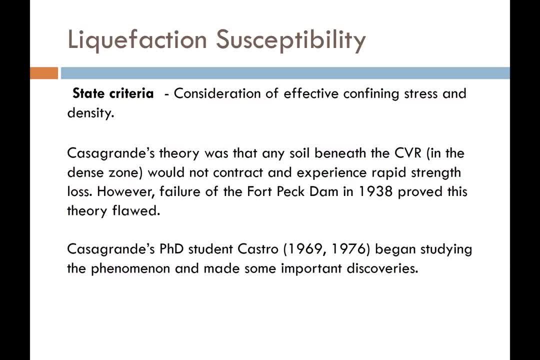 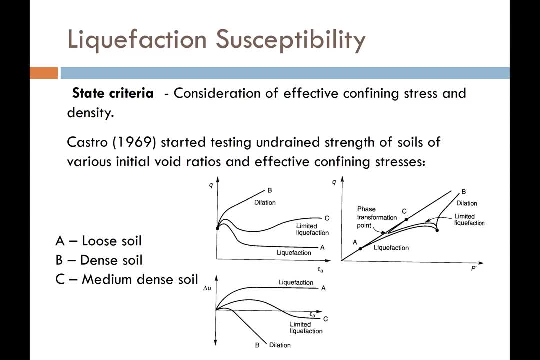 in 1969 and then later in 1976, published some of the results from his PhD work And he made a few important discoveries. He started testing the undrained strength of soils At various Initial void ratios and effective confining stresses. 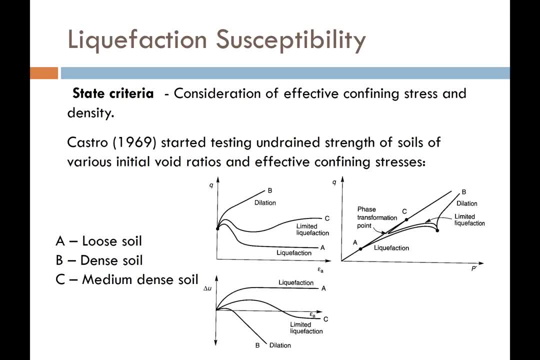 And here's some of the things he found. Let's say, what I have here is I have stress paths. Oh, actually, whoops, I'm sorry. This is the stress path, This is the stress strain curve And we have a pore pressure versus strain curve down here. 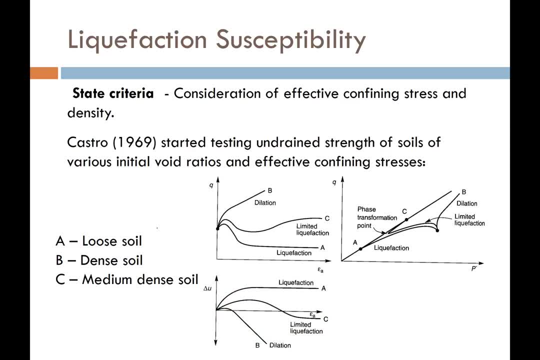 And all of them are plotting the paths for these three different soils that Casa Grande was testing, And so what we saw, for instance, for a loose soil, is something that we would totally expect. For the loose soil, we'd expect to see a little bit of strain, hardening and then a sudden 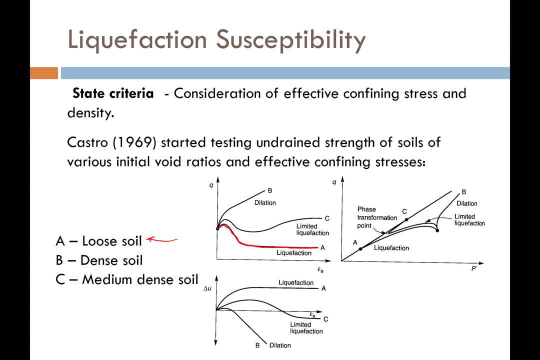 drop in our strength and then huge strains. That corresponds with a stress path that drops dramatically and approaches the failure envelope at point A And in turn we see a drop in our strength And in turn the pore pressure, the excess pore pressure, because it's loose and contractive. 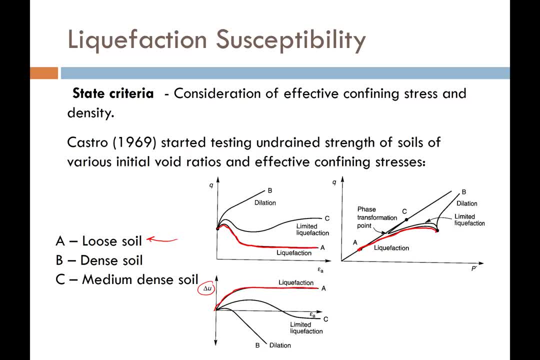 we expect to see a big increase in our excess pore pressures during that process. So that's a soil that liquefied. Now, if we look at soil B, that's a dense soil. This is a soil we'd expect to dilate, meaning that it's going to gain strength with strain. 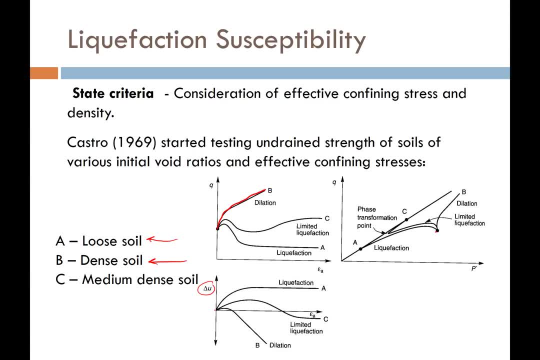 because of the vacuum effect and the negative pore pressures that generate strain. So that's a soil that liquefied. Now, if we look at soil B, that's a dense soil. This is a soil we'd expect to dilate during shear. 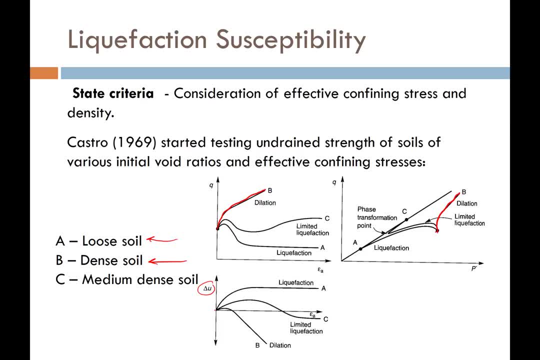 And because of that my stress path goes to the right, not to the left. Whenever I have dilation, my stress path goes to the right. If I have contraction, my stress path goes to the left, And then I get a little bit of initial increase in my pore pressure and then my pore pressure. 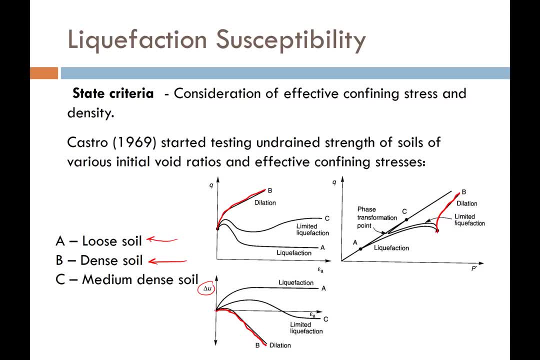 goes negative, creating a vacuum and suction within my soil that adds to it an additional or a false sense of strength. So that's a soil that liquefied. So that's soil B. Now soil C is what we call a medium-dense soil and it's something between: 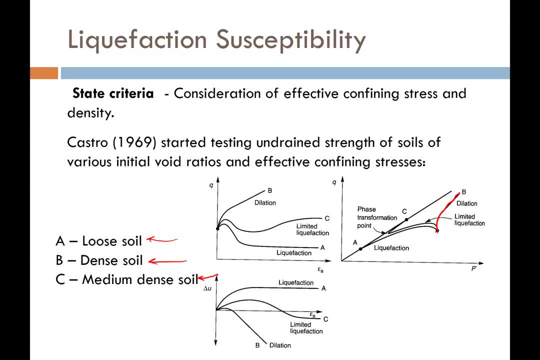 the loose soil of A and the dense soil of B. And this is where Castro saw some interesting behavior. He saw, for instance, some initial strain hardening and then it started to strain, soften like the liquefied soil, But then it started to dilate and harden like the dilative soil. 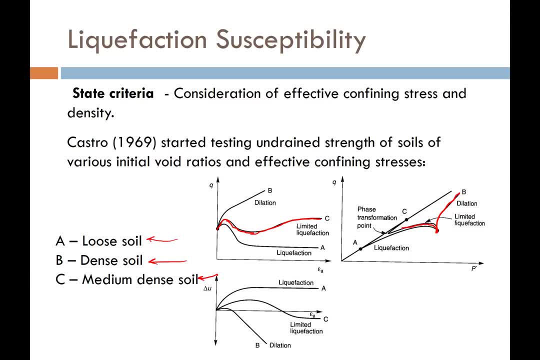 In terms of stress paths. It again softened and then had a sudden change in direction and it started to dilate until it hit the failure envelope of point C, And he called that point the phase transformation point. That's the point where the stress path changes direction abruptly. 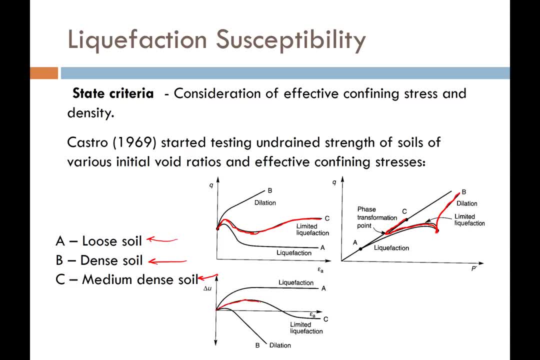 In terms of pore pressures, there was a slight increase initially, as the soil began to soften, But then it went negative as the soil began to dilate, And so Casagrande referred to this term as limited liquefaction. We don't really use that terminology today. 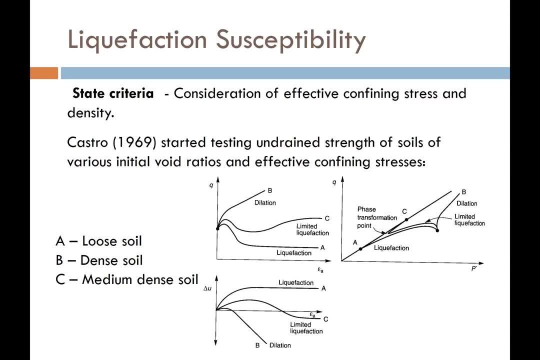 What we know is that all soils tend to show some contractive behaviors if they're loaded long enough or loaded at a high enough amplitude. But this limited liquefaction behavior just is the behavior of soil that is, between a loose and a dense soil. So I want to point out this one point here, where the liquefied soil dives to 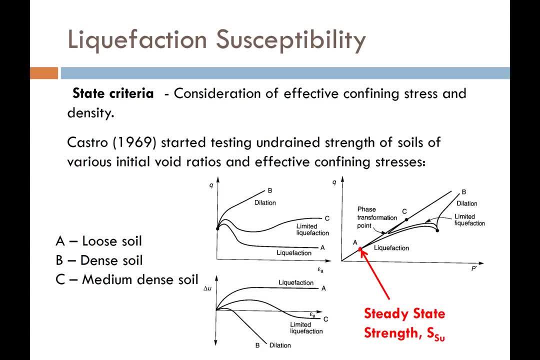 When the soil liquefies and it jumps down and hits the failure envelope, it's going to hit it at what we call the steady state strength And we call that strength S of SU, And think of this as the residual shear strength for the liquefied soil. 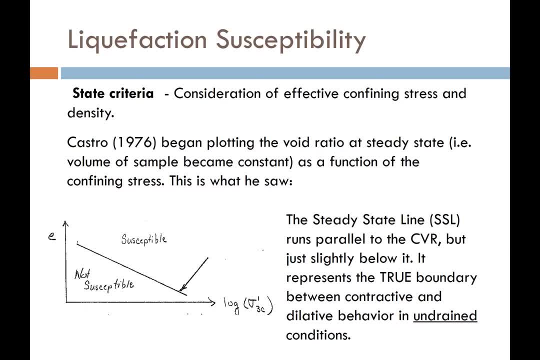 So what Castro started doing is begin plotting the void ratio of the soil At the steady state, I mean, in other words, after the soil hit that steady state, strength on the failure envelope. And what he noticed was that a couple of things. 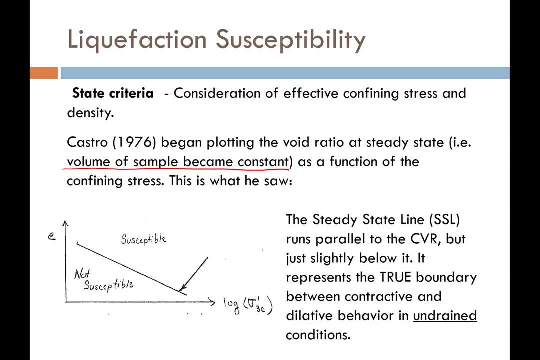 First of all, the volume of the sample became constant. Its void ratio wasn't changing anymore once it reached that steady state- Even though we know that it was still an undrained test- And so what he saw when he started plotting This behavior was what we call the steady state line. 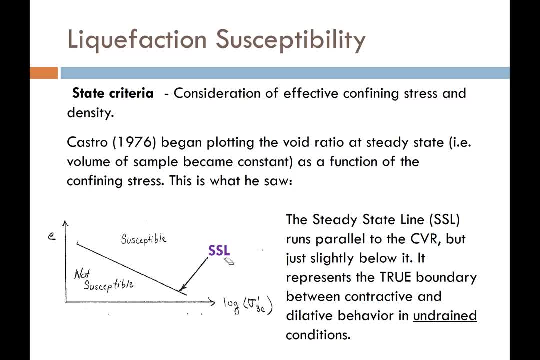 And it's very similar to the critical void ratio line that his PhD advisor had discovered decades before. But it's not the same line. In fact it lies just slightly below it, And it represents the true or the actual boundary between contractive and dilated behavior under undrained shearing conditions. 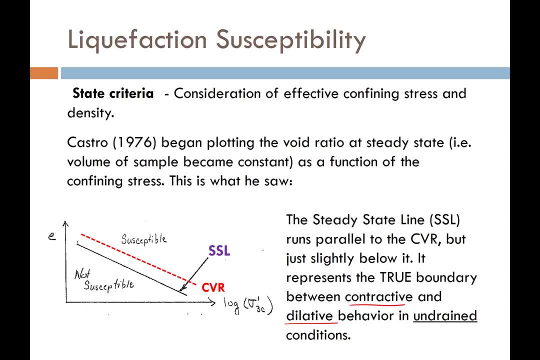 See what went wrong with With Casagrande's work was back in the 1930s. We really didn't have a good way to perform undrained shear tests, And so his theory was solely developed based on well theory. 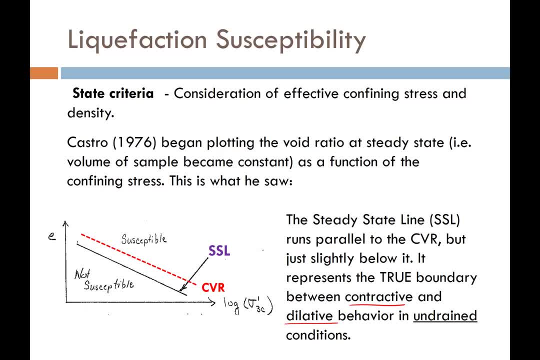 But it didn't have any testing to back it up. And so Castro's work is so important, because now we're able to show that if you test the soil in an undrained manner, It almost shifts the critical void ratio line, And we 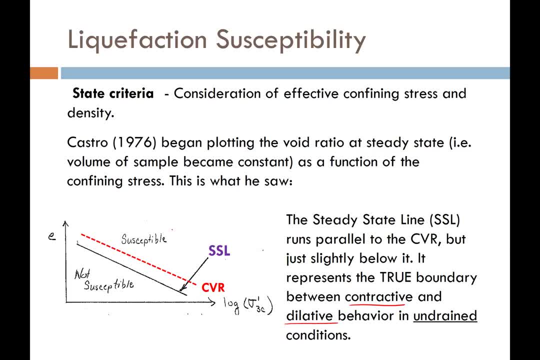 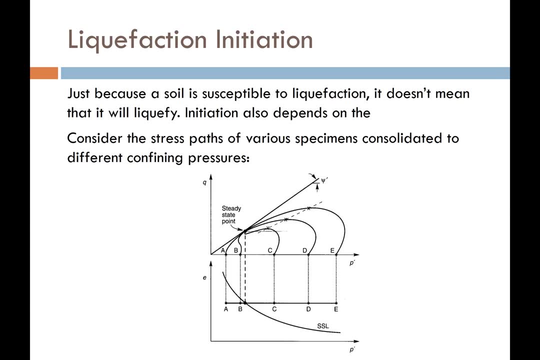 We use, then, that steady state line to tell us whether a soil is contractive, And in other words susceptible to liquefaction, or dilative, And in other words not susceptible to liquefaction. So that wraps up everything we need to talk about with susceptibility. 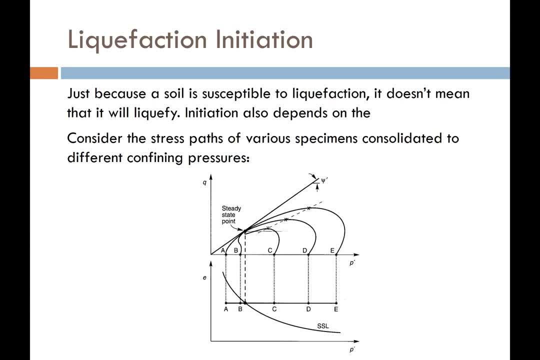 So, again, an engineer would look at soil and would ask the question: is this soil susceptible to liquefaction? And they could look at historic, geologic, compositional and state criteria to try to answer that question. Now, if the answer to that question is yes, the soil is susceptible to liquefaction. 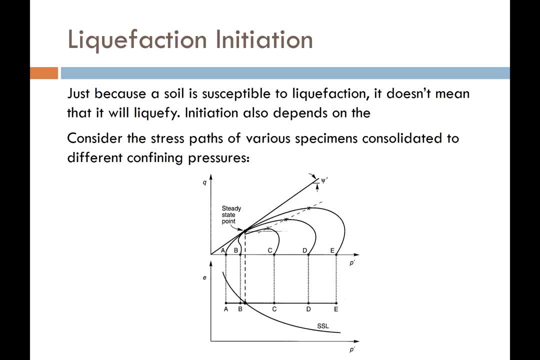 Now, it doesn't necessarily mean that the soil will liquefy for sure if exposed to an earthquake, And that's because the initiation of liquefaction also depends on the magnitude and the duration of the loading that we apply to the soil. So consider the stress paths that are shown in these plots below. 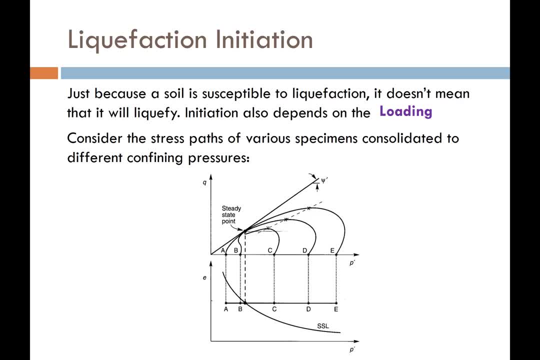 What we have is five specimens of soil, all prepared at the same relative density, But all we're doing is consolidating them and shearing them in an undrained manner at different confining stresses. As such, you can see that some of these soils plot. 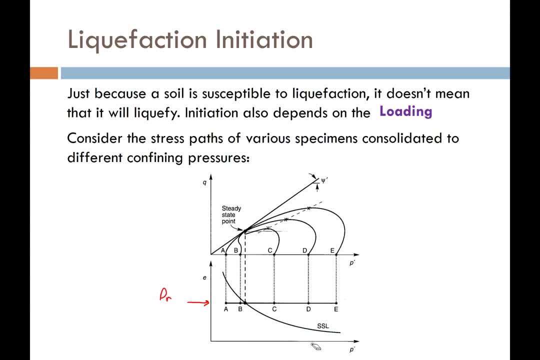 Below the steady state line And some of these soils plot above the steady state line, which means that the soils on top are contractive And the soils below are dilative. Now if I start loading say soil C up, I can load it, load it, load it monotonically. 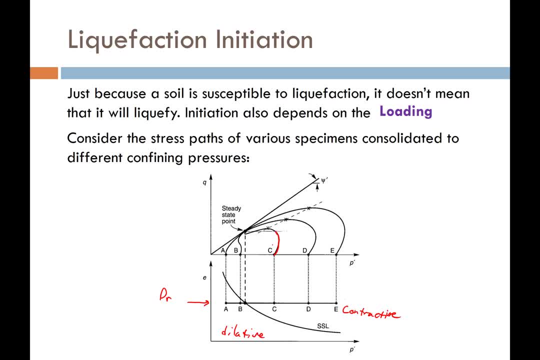 And if I were to stop at any time, the soil would be fine. But if I were to load it up to a certain depth, that'll be fine, But those soils will be good. Soil which are basically is higher than, for example, solid. If I had to load my soil over that depth, I'm Vericking my soil and that would be perfect and perfect and identical. So that's a good second to do that. And then we're going to do some demystification of protruding soil. 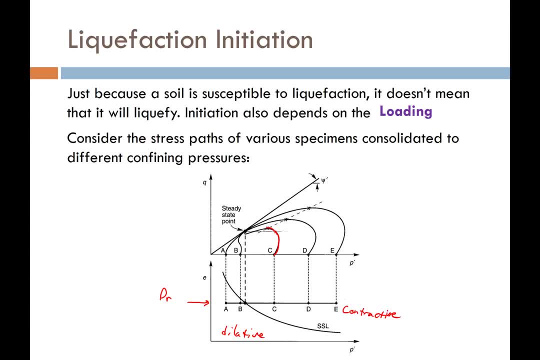 certain point. at that point, once it reaches a certain point, there's no stopping it. It just flies down to the steady state strength and resides there. The same with soil D. If I load the soil D up- and I keep loading it up, the effective stress path starts moving to the left. 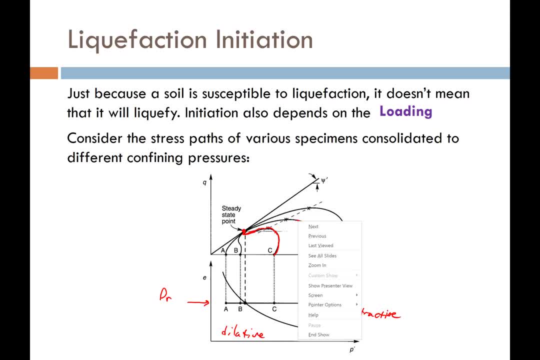 because of positive pore pressures due to contraction of the soil. Eventually it hits a point where it just dives to the steady state strength, Same with soil E. Once it hits that point, it just dives to the steady state strength. Conversely, if I have soil A, if I load, 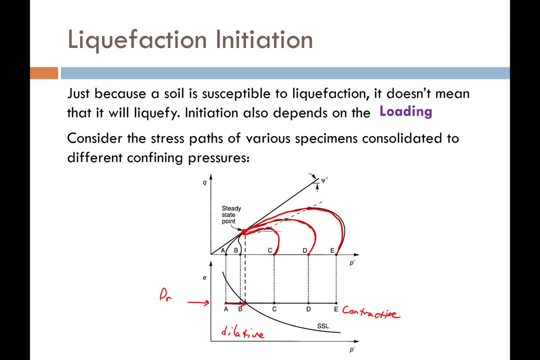 soil A up. it has to go to the right in terms of a stress path, which means, then, that as it goes to the right- that implies dilation- It's also going to travel to the steady state point. All of these paths are flying to the steady state point. The only difference is: 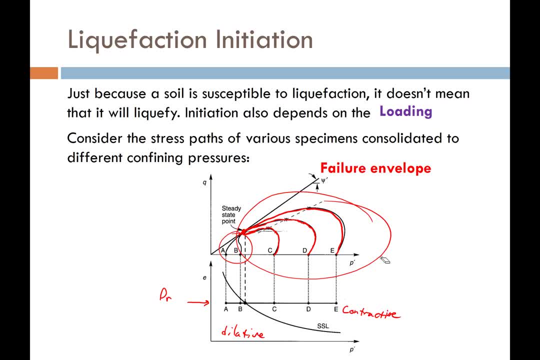 these three soils right here- C, D and E- reach the point where there was no going back. Once they reach that certain critical point, the strength of the soils degraded rapidly and there was no stopping it. In fact, if we were to take that, I've got a little bit. 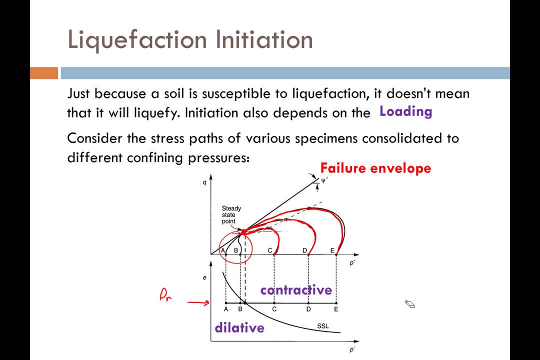 of labels there that popped up. If we were to take the point of no return for each of those stress paths, we could plot a line through those points. We can call that line the flow liquefaction surface. The flow liquefaction surface defines the line or the surface. 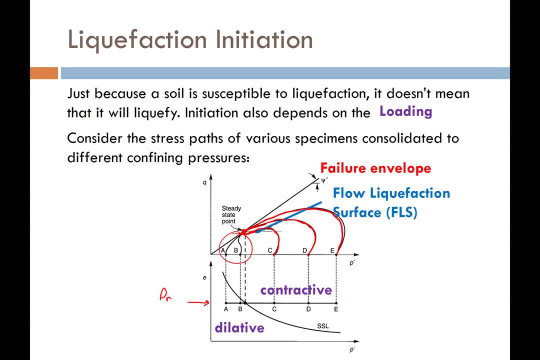 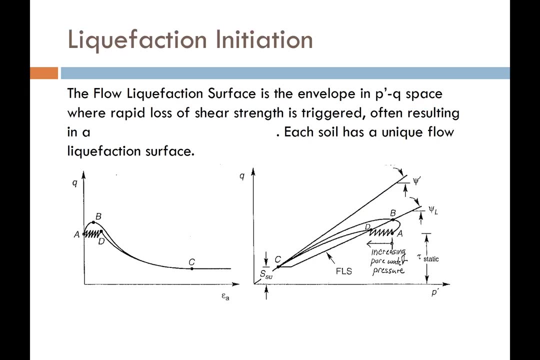 if you want to think of it that way, where, if the stress path hits it, flow liquefaction is initiated and the stress path rapidly dives to the steady state strength or the steady state point on the failure envelope. Now the flow liquefaction surface is the 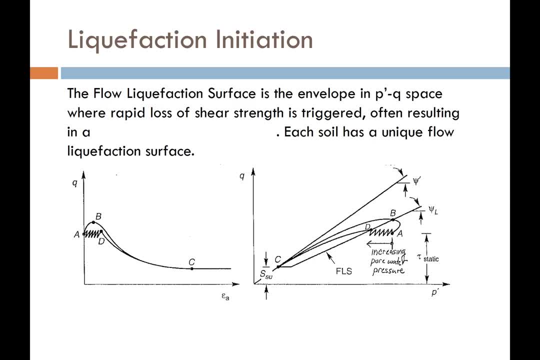 envelope in PQ space where rapid loss of shear strength is initiated or triggered, This will often result in a liquefaction. In fact, it also causes a liquid action flow failure if the soil is unable to hold up its own weight at that point. Each soil has its own unique flow liquefaction surface that 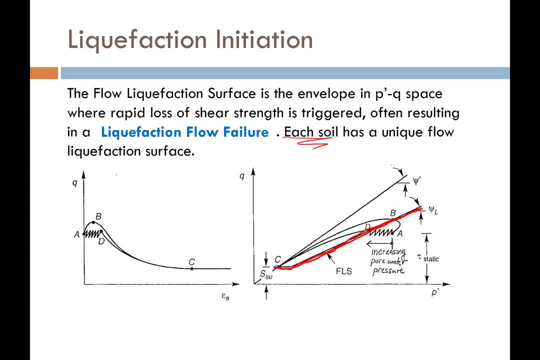 can be identified through shear testing in the laboratory: The angle of that flow liquefaction surface. we can call it psi sub L. All we know is that whenever the soil is not in a, whenever the stress path of our soil hits that surface, it will initiate flow and the soil will. 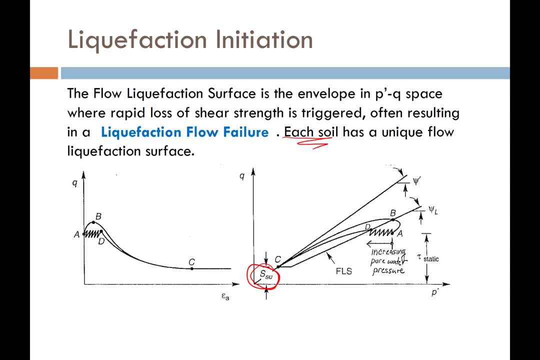 rapidly reduce its strength to the steady state strength. Now, in terms of these different stress paths, if I look at stress path A and B, this is just from monotonic static loading. As I load the soil monotonically, positive pore pressures start to generate which cause my stress path to bend and 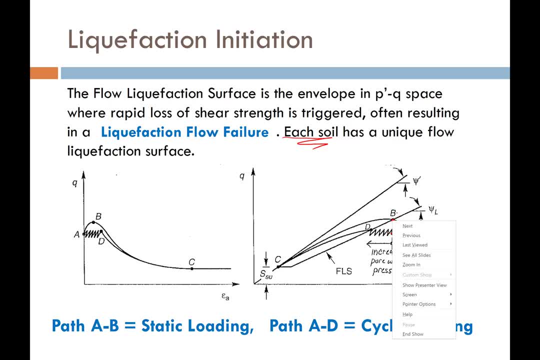 move to the left. Once it hits the flow liquefaction surface at point B, it dives rapidly down to the steady state strength. Conversely, I can also get there if I do cyclic loading. So if I'm at the same starting point and I start to load my soil cyclically, every cycle generates pore pressure. 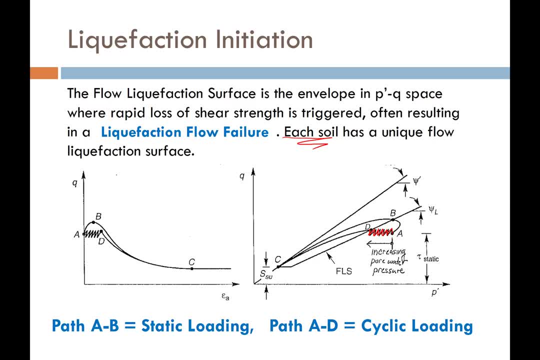 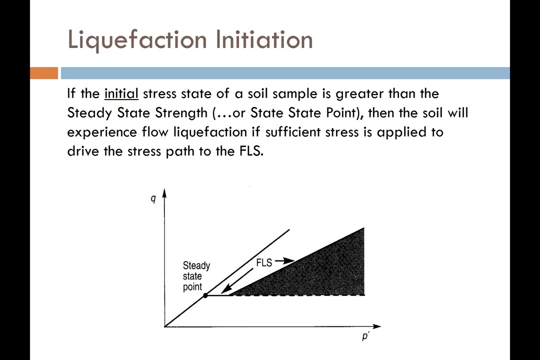 An excess pore pressure causes my confining stress to reduce. so my stress path starts moving to the left. Eventually it ratchets itself and will hit point D on the flow liquefaction surface, and then it dives down to the steady state strength. So what does this mean then? Well, it means that if my initial stress 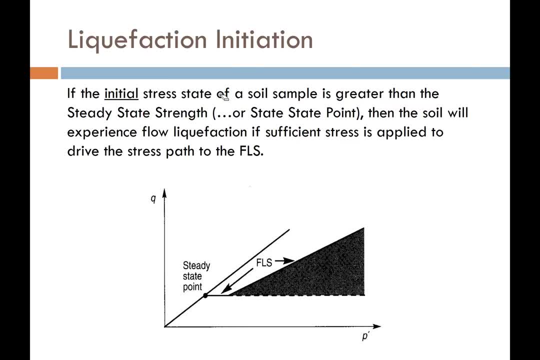 state of the soil is greater than the steady state strength which is located right there, then the soil will experience flow liquefaction if sufficient stress is applied to drive the stress path to my flow liquefaction surface. So all this region that's shaded here is the region where a soil is susceptible to flow. 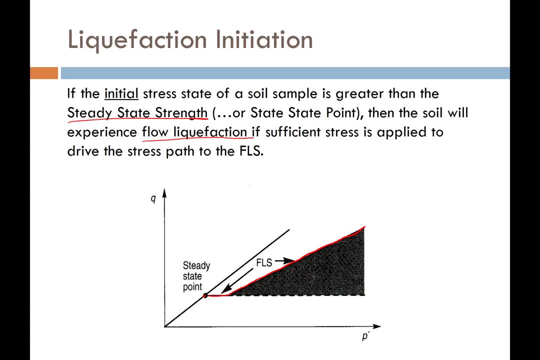 liquefaction And if the stress path of that soil ever hits point B, it's going to hit point C, which is going to hit that flow liquefaction surface. it will trigger flow liquefaction and you'll see a rapid and unstoppable reduction in the soil shear strength. 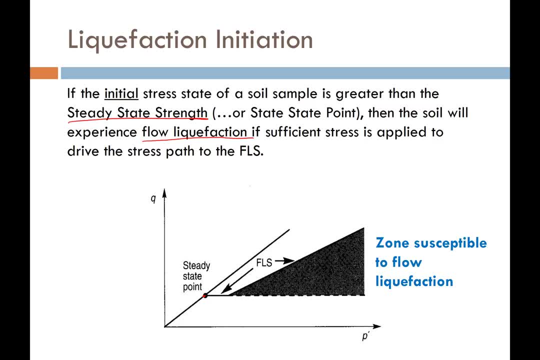 So we then would call this zone the zone susceptible to flow liquefaction. But what if? what about this stuff down here? What if my, what if my soil's initial stress state is down here and I start wanting to load it up either cyclically, or I want to load it up monotonically. 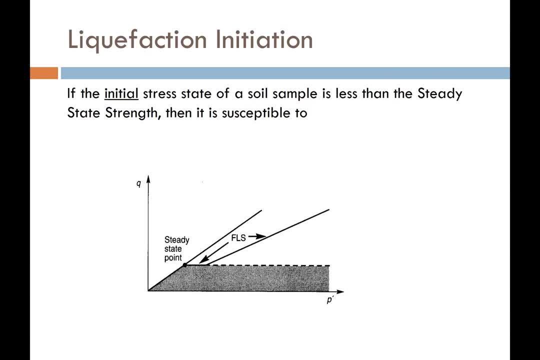 Well, if that's the case, then we have a soil that is susceptible to cyclic mobility. If the initial stress state of the soil is down here, the initial stress state is already less than the steady state strength. So what that means is that if my soil ever makes it to the steady state strength, 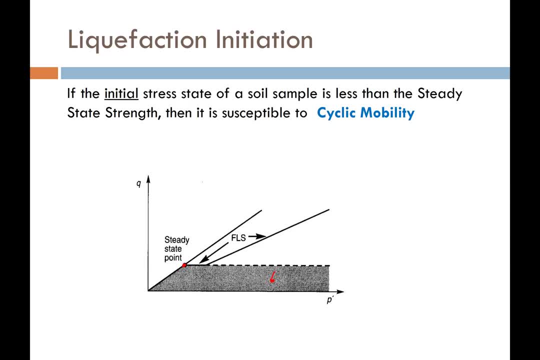 well guess what? It's a gain in strength, because that point is higher than my initial stress. So we don't have a sudden or a drastic drop in strength. But what we get with cyclic mobility is the ability to ratchet back and forth, back and forth, until we eventually make our way to the failure envelope. 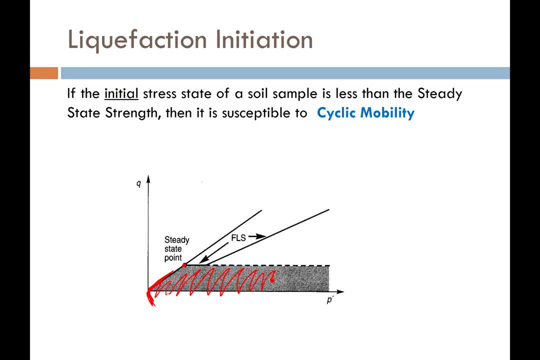 And then we start diving back and forth on the failure envelope with every cycle of our loading. So this region that's shaded here is the region that is susceptible to cyclic mobility. It's important that you guys know these two regions, both the region susceptible to flow liquefaction and the region susceptible to cyclic mobility. 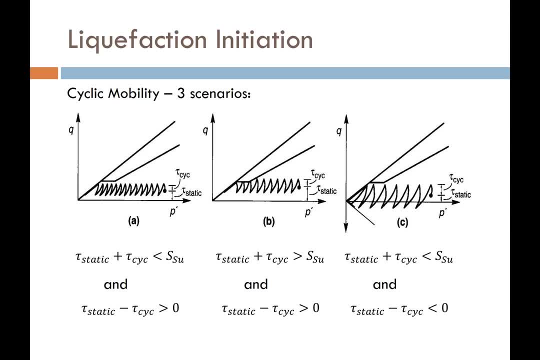 Now let's just give you three scenarios of how cyclic mobility might initiate. The first scenario is our initial shear stress in the soil plus the shear stress from the earthquake is less than our undrained or our steady state shear strength And the difference between our initial shear strength and the static or, I'm sorry, the initial shear stress and the shear stress. 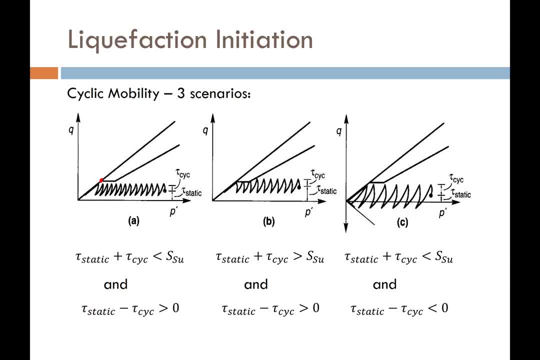 induced by the earthquake is greater than zero. What that means is my cycles, my stress path, is staying on the positive side And in this scenario it's going to take a lot of cycles to get all the way back until I fail on the failure envelope, and then 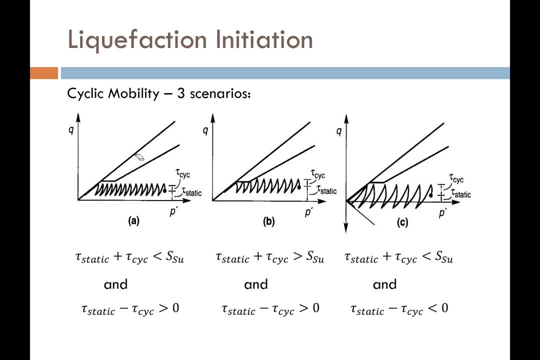 I just go back and forth along the failure envelope. Now scenario b. It's similar to the first one, with the exception that my initial shear stress plus the shear stress from my earthquake is greater than my steady state shear strength, undrained strength. so, in other words, as I come up each one of these peaks, if I 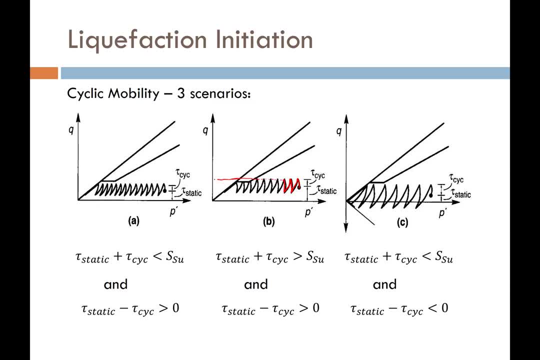 were to come over is larger than my steady state strength right there, and so that eventually means that my stress path is going to hit the flow liquefaction surface, but right at the bottom. but it doesn't really do anything. all it does is accelerate the strain in these little regions where the stress 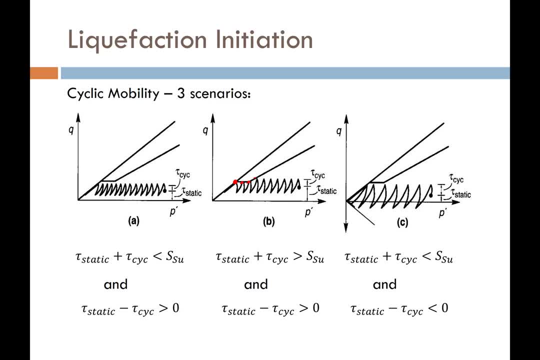 path hits that surface, but we don't have catastrophic losses of strength, and the reason for that, again, is because my initial stress is less than my steady state stress. the third example is an interesting one. it's where the initial shear stress plus the shear stress induced by the earthquake is less than. 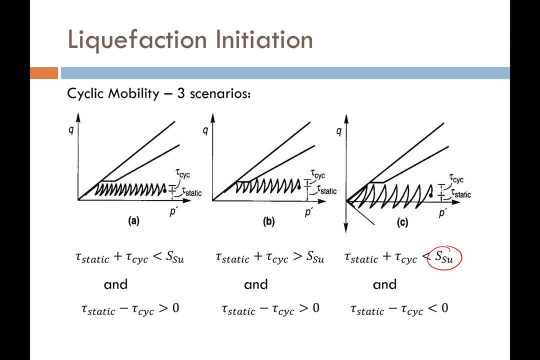 the initial or the steady state strength of the soil, but the initial stress minus the stress of the earthquake is less than zero and what that means is that my stress path has a stress reversal where it's positive and then it goes negative temporarily, and then goes positive and then goes negative again. whenever I have 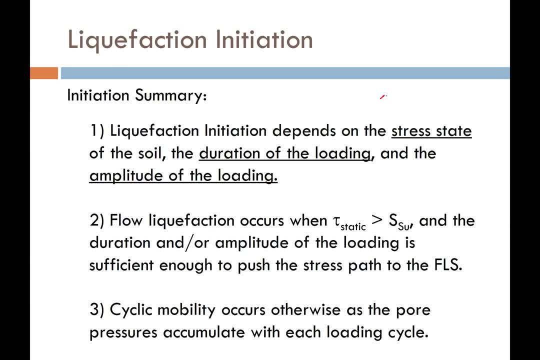 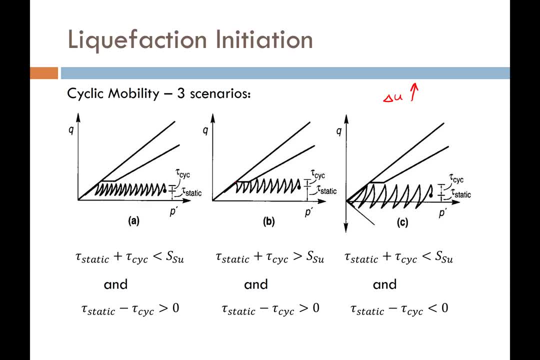 a stress reversal that really increases the change in my effective stress and my excess, I'm sorry. it increases the excess poor water pressure and a change in that excess poor water pressure and so it accelerates the onset of liquefaction whenever we have those stress reversals. 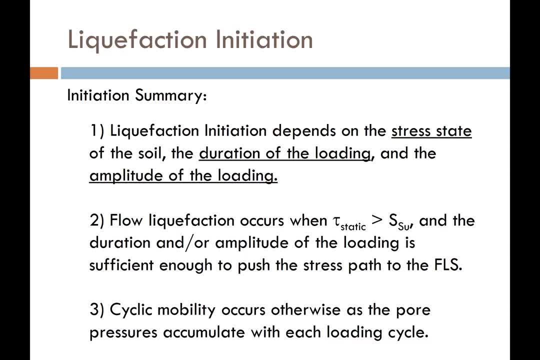 so let's review a couple things about liquefaction initiation. we know that the is going to depend on the stress state whether or not the soil is contractive or dilative, and that depends on its location relative to the steady state line. if my initial stress state is above the steady state line that my soil is. 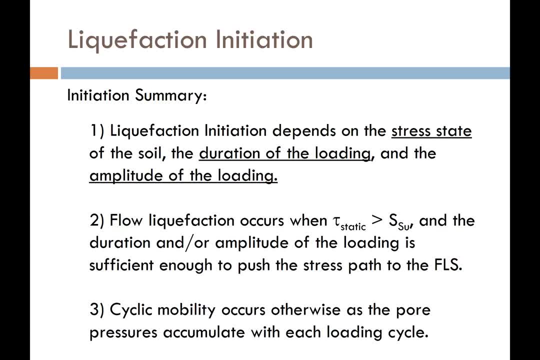 contractive. if my steady or my initial stress state is below the steady state line that my soil is dilated. now it also depends on the duration of the loading. if I have enough cycles I can move my way all the way to the left, over to the failure envelope, and it also depends upon the amplitude of my loading. 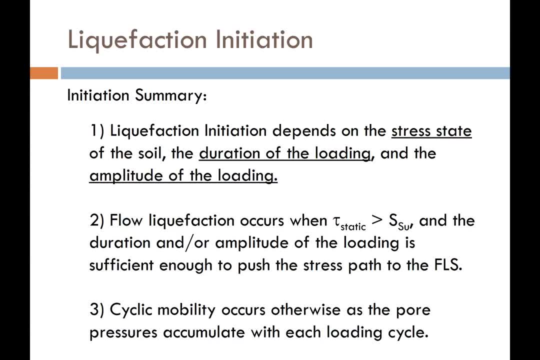 if my amplitude is large enough that I can actually introduce some stress reversals in my stress path, then we can really accelerate the loading of the soil and then we can actually move my soil to the right and accelerate the generation of pore pressures. now we know that flow. 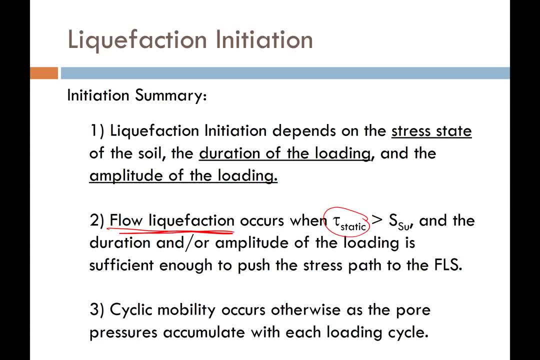 liquefaction occurs when the initial shear stress in the soil is greater than the steady state, undrained strength of the soil and the duration or the amplitude of the loading is sufficient enough to push the stress path of the soil to touch the flow liquefaction surface. if that happens, flow